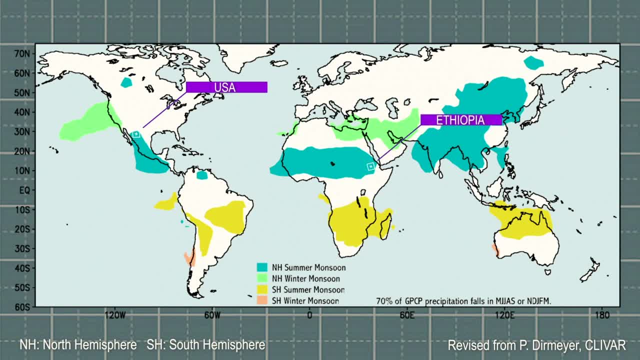 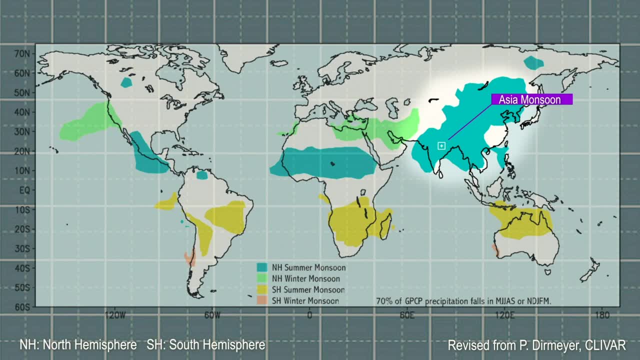 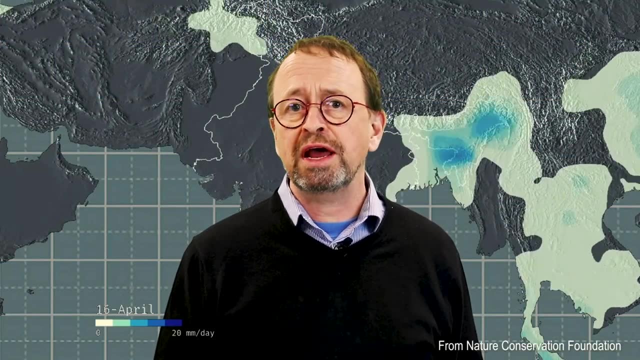 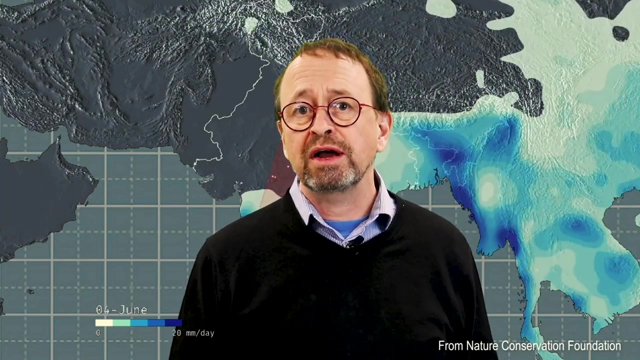 something like monsoon, as does Ethiopia. Asia just has the strongest, most important and most famous monsoon. So where is the monsoon, Although a monsoon can occur anywhere between a large continent next to a warm sea. for the remainder of this video, when I talk about 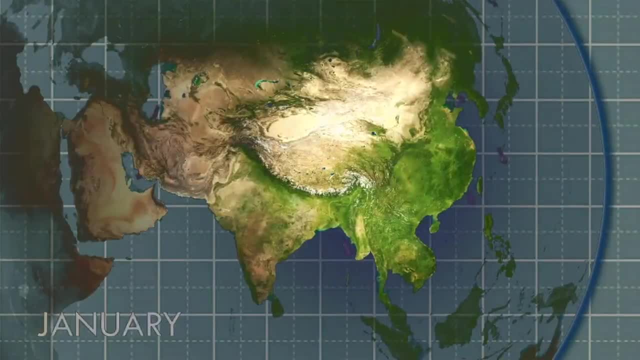 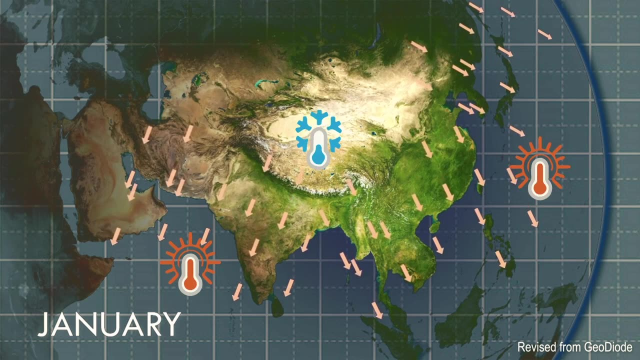 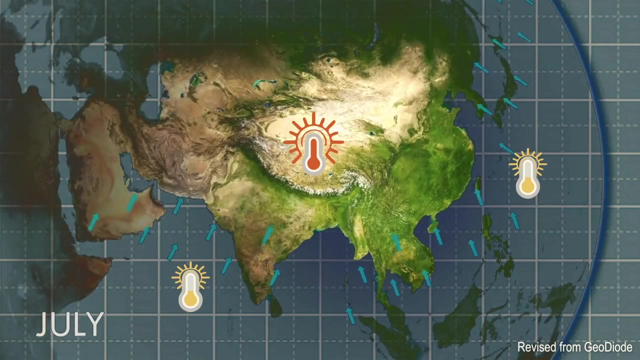 the monsoon, I mean the Asian monsoon. Okay, what happens with monsoon winds in Asia? It's simple. They blow out of cold, dry Asia towards the Indian and Pacific Oceans in the winter and from the warm, wet Indian and. 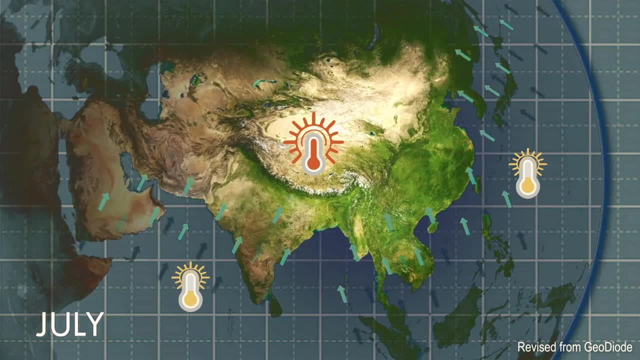 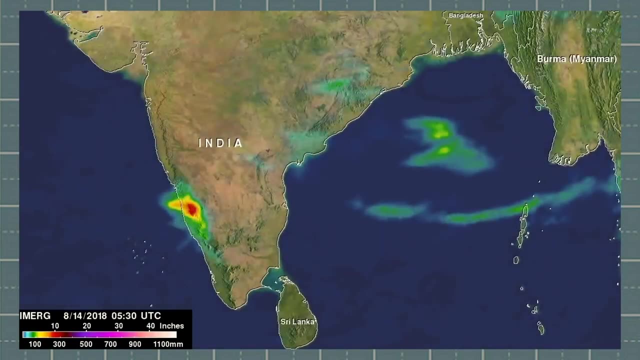 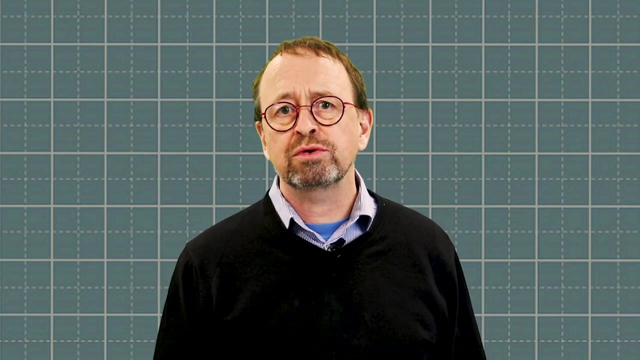 Pacific Oceans towards the continent. in the summer, The summer winds bring rainfall deep into the continental interior and not just along the coast, as seen in this video. So why is the monsoon important? The winter monsoon is not so important, but the summer monsoon. 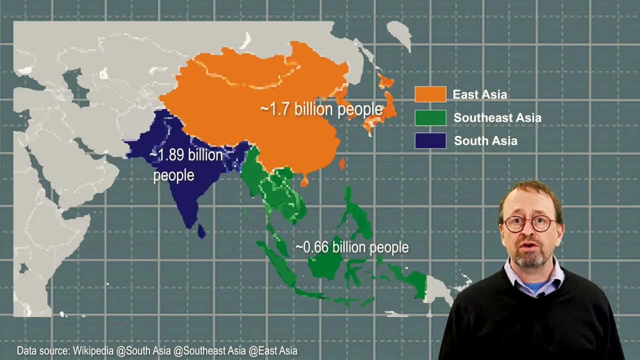 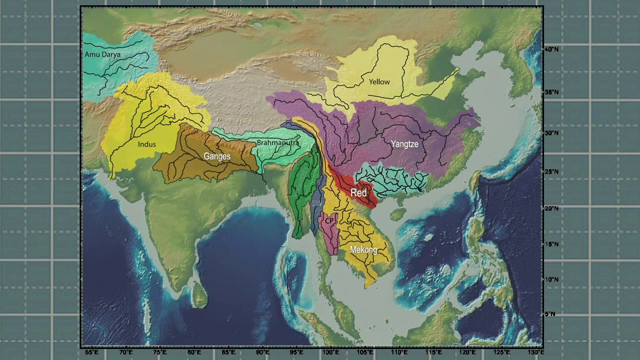 rains are the single most important feature, controlling and allowing agriculture across much of the densely populated regions of South Southeast Asia and Eastern Asia. The summer monsoon also supplies water to the great river systems that flow out of the Himalayan highlands, including the Indus, Ganges, Brahmaputra, Mekong, Red, Yangtze and 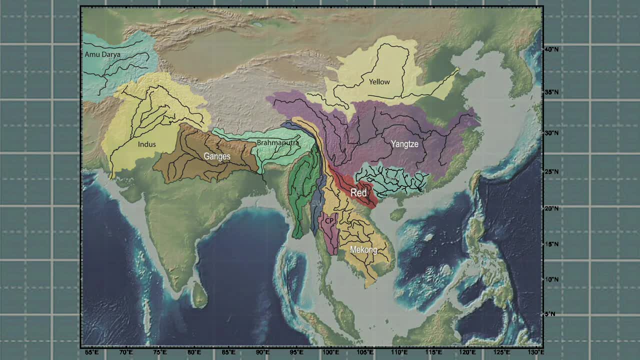 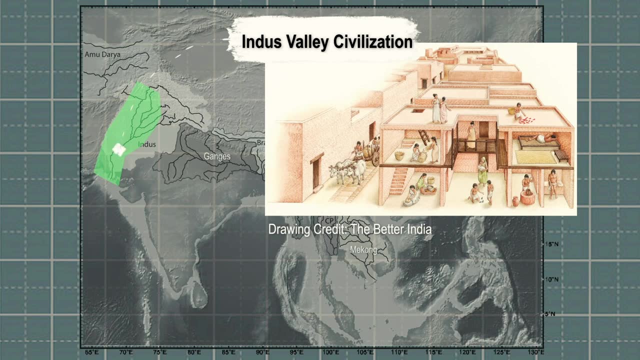 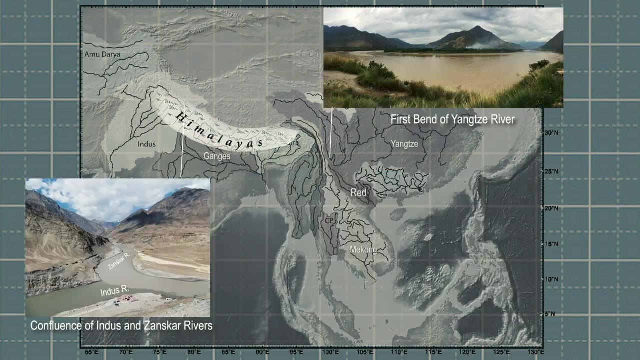 Yellow rivers. Many early civilizations started in these river valleys, such as the Harappan or Indus Valley culture. The rainfall is also important in sculpting the mountains of Asia, especially the Himalaya, and erosion provides detritus that covers the floodplain and the. 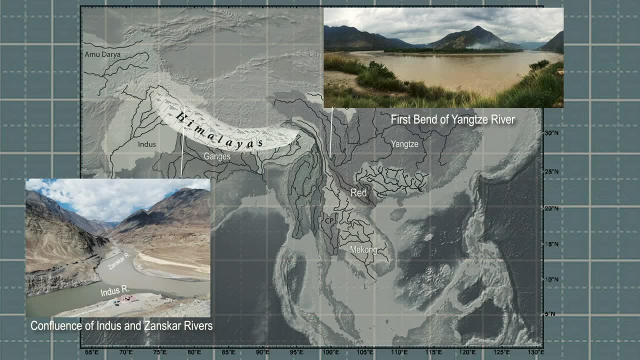 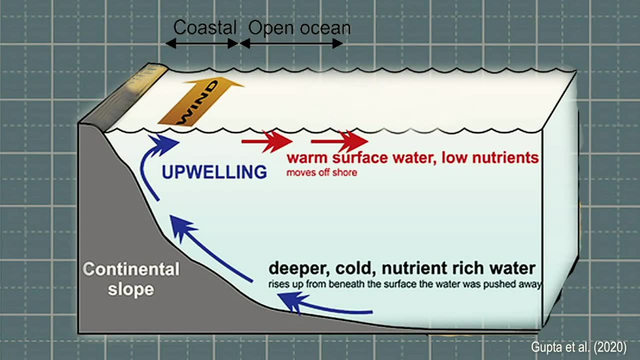 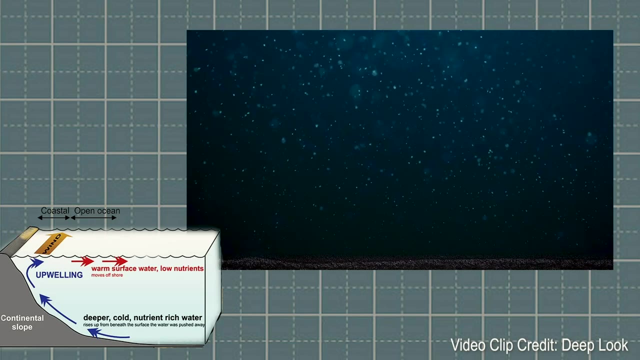 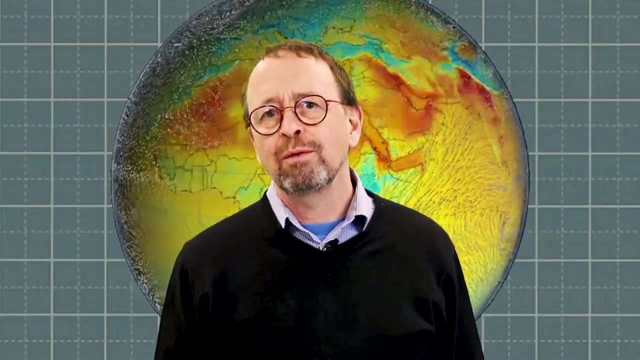 deltas of these rivers, quickly becoming fertile soil for agriculture. The winds are also important in causing upwelling of nutrient-rich seawater adjacent to coastal regions, allowing fish and other marine life to thrive. How does the monsoon work? What causes the monsoon?